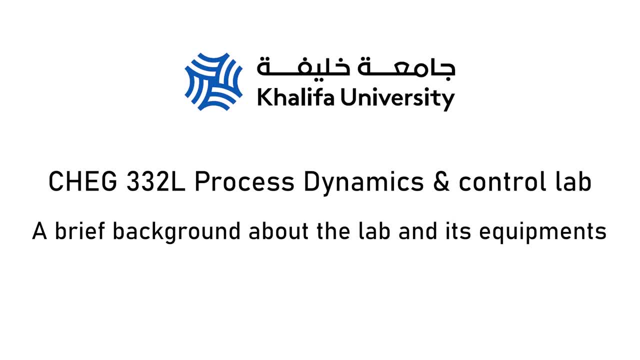 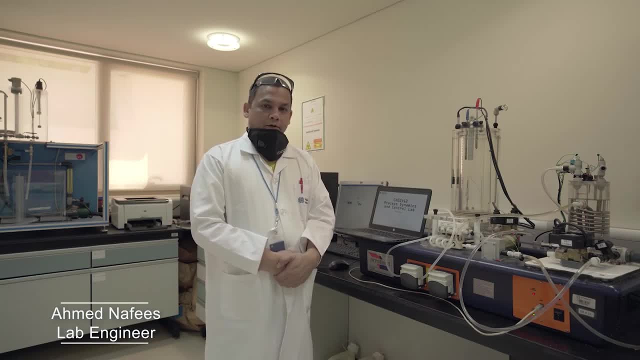 Assalamu alaikum and welcome to the Process Dynamics and Control Lab. We are in the lab here because we want to do the experimental part of the lab. As you know, the lab is in three parts: First part: we do the MATLAB. second part, we do the Simulink. and third part. 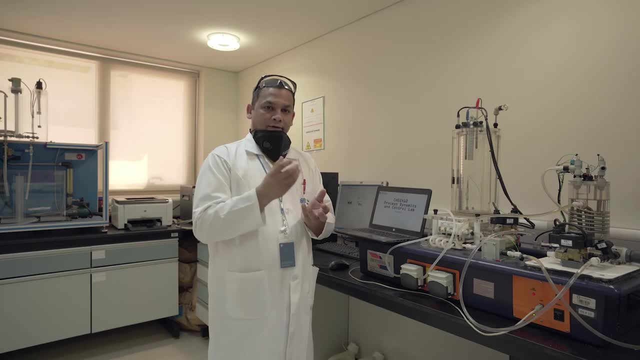 is the experimental part. So all of the three parts. you can do all the activities that you need. and what is the activity? You want to study the controller and you want to find out what is the best value for the controller. that will give you a better control on your parameters, Whenever. 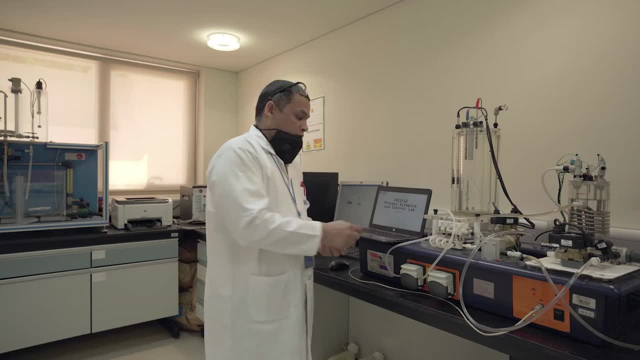 you apply a disturbance, how the controller will behave. So we are studying the process, three experiments in the experiment part. here We are doing the level control in the tank. here We are doing the temperature control as well as we are doing the flow control. So just a little bit. 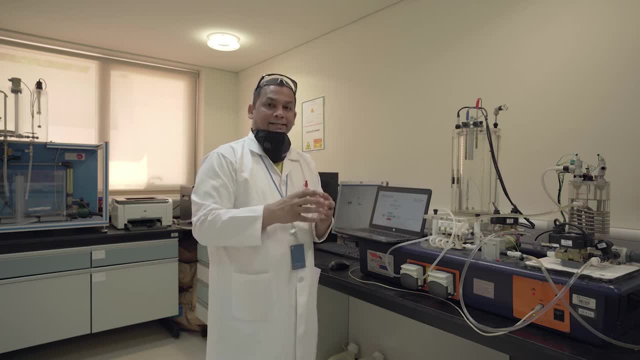 of the background. We all know that in the feedback controller there are certain elements that are there to do the job, And the first element is always the measurement or the measuring device. So in the case of temperature, it will be a thermocouple, in case of pressure it will be a 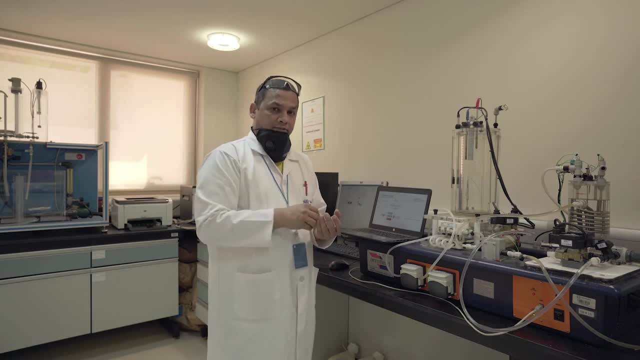 differential pressure, or it may be a height measuring device or, in case some other experiment you are doing, it will be on the device. So you have measuring device, then you are comparing the value with your set point and then you are calculating the error. Error then signal, you are. 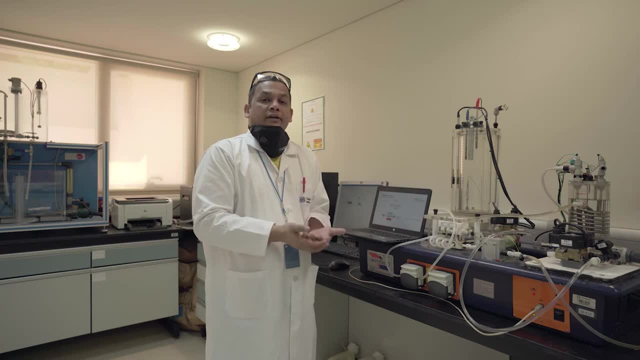 providing to the controller. then controller decide what need to be done, what correction to be done so that set point can be maintained, And how it do that one using a finite final element, which may be a control valve, which may be a temperature power control or something else. Okay, so this is the 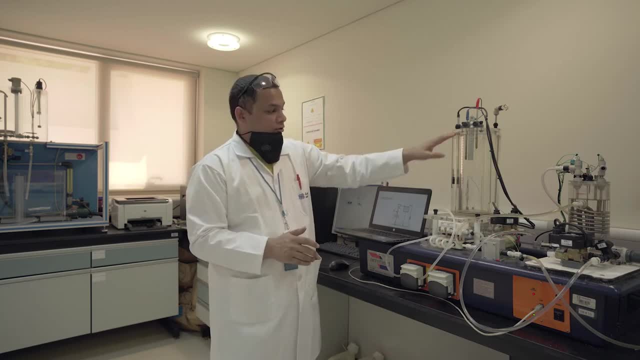 level control. The first experiment we do, the simplest one, which is the level control. In this one I want to maintain a desired level, So I will put in the controller my desired set point and then I will switch on the controller in automatic mode with the controller values, the PID settings. 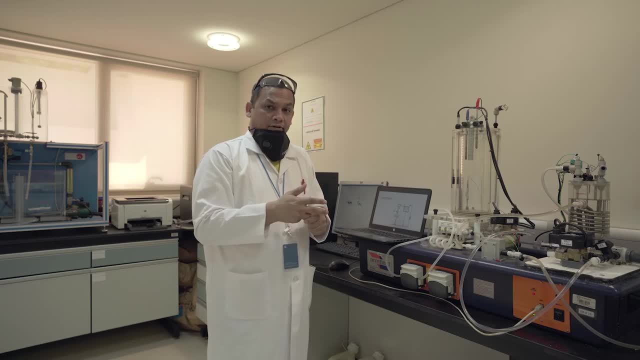 which are proportional value time, the integral time and the derivative time, so that the controller tries to minimize the impact of the disturbance in the system and try to reach the set point. So the same is here in the case of temperature. You have a thermocouple connected to the tank. here you measure. 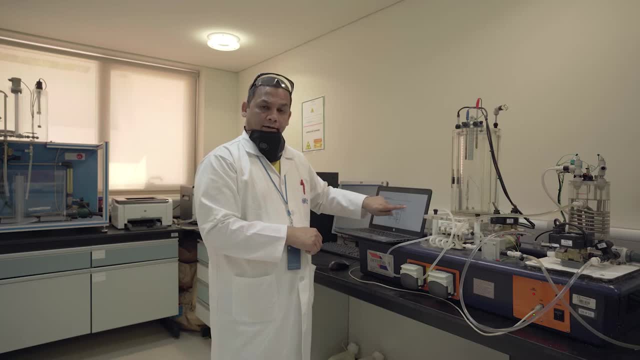 the temperature and then compare with the set point, calculate the error, send it to the controller and then the the final element, which is the hot water supply here in this case, tries to reach the set point. The third experiment is the pressure, the flow control that you want. you want to maintain a flow rate, a desired 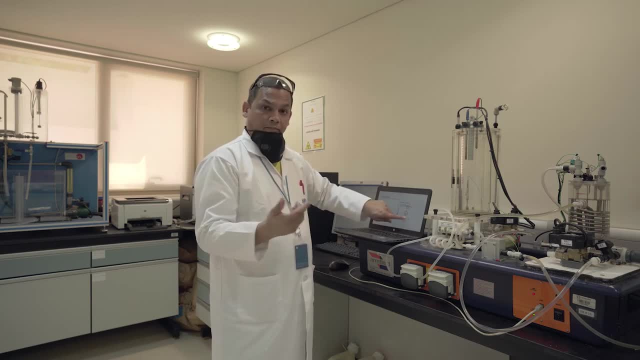 flow rate. So you measure using an orifice meter here. The orifice meter then send it to the comparison with the set point and error, go to the controller. controller then decide what need to be done. Should the valve need to open more or should decrease the more? 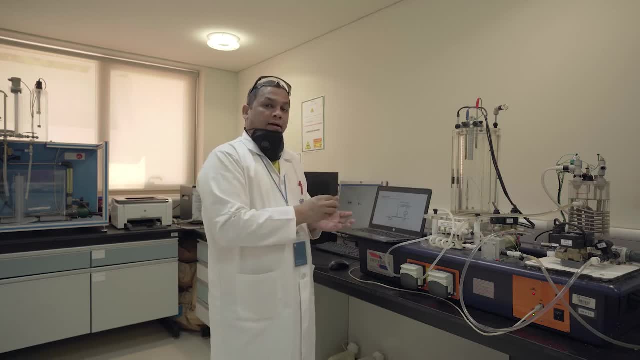 So all the three, So all the three, So all the three experiment that we do here. you can see the controller can act or can work on. in the tank you have an inflow or outflow, so either you can manipulate your inlet flow or you can manipulate the outlet flow. any one of them, you need one at a. 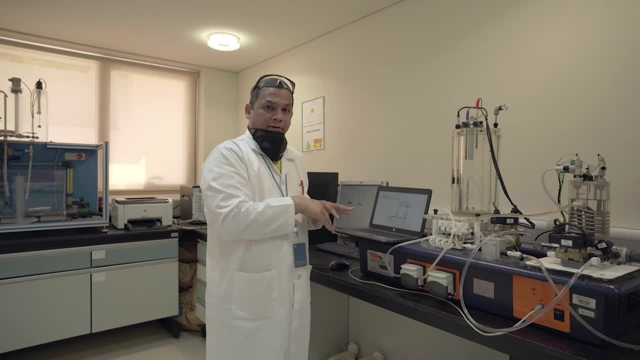 time you don't need. so the experiment will be done in two part. for all the three experiment that we do in this lab, you are doing first inlet as a manipulative variable, then outlet as manipulative variable. okay, so what kind of experiment or the activity that you do? now we know that the controller it. 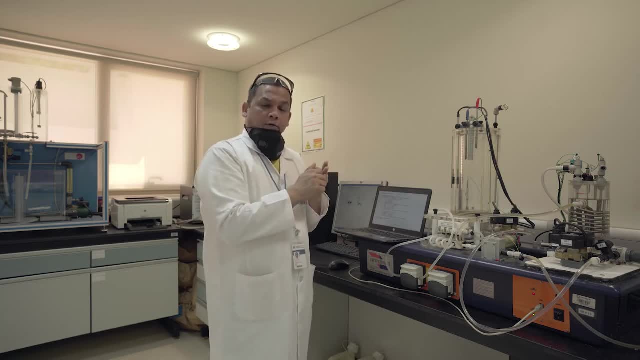 basically have three settings: the P, I and D. so what I need to do is first and first thing that I need to do is I need to understand how the P value will impact my controller, how the I will, where the control will have impact on my controller. the D will have impact on my controller. so P individually I need to 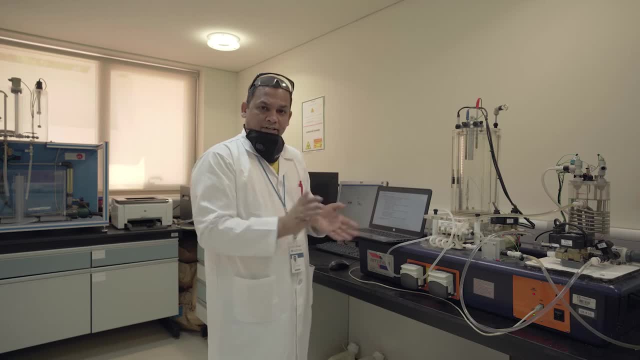 do so in each of the three experiment. the procedure is very similar. first, I want to put the value of the integral time and derivative time zero. only change the P value three, four different times so that I can see the impact of the P on my controller setting: whether it's better when the P value is small, whether it's 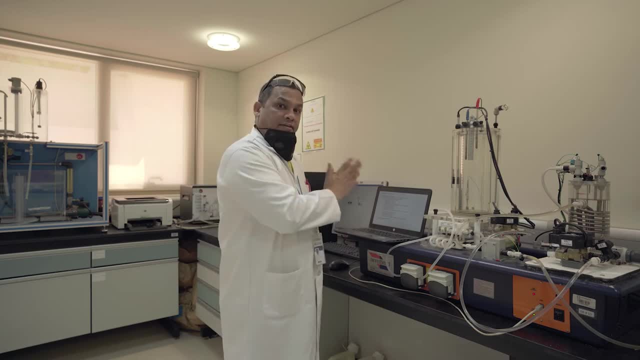 better. when the P value is large, like that, then I will fix the P value and I will now keep the D value zero and I will change the I value- different, three, four times different, different integral time- and see the same thing that if I increase the I value but it is better if I keep. 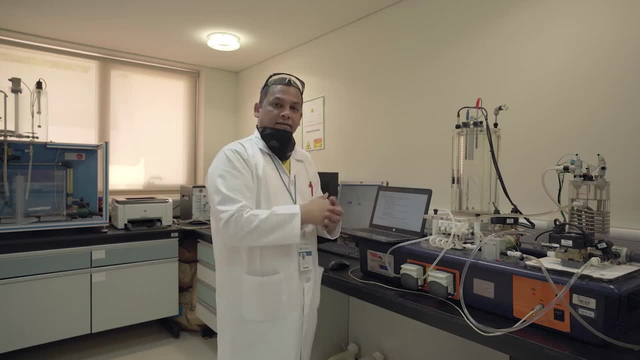 the low if I keep high, whether it increasing or decreasing and so on. so I studied the impact of the P. I should be back up I now I will study the impact of the D. so when I am doing the D I will keep a fixed value of P and fix a low. I. 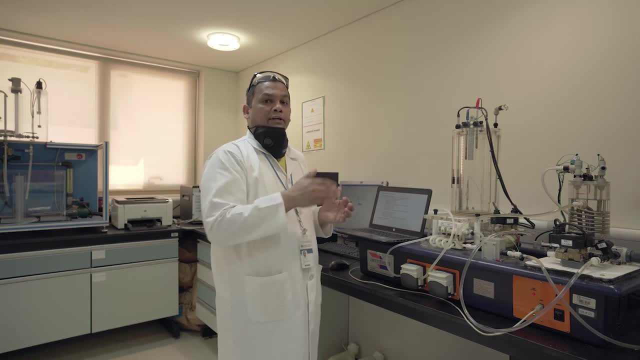 and then change the value of the D three to four different times and plot them together to get the idea how the D will impact. so from this is like I have to do it for the when the inlet is manipulative variable and outlet manipulative variable. so this is the. 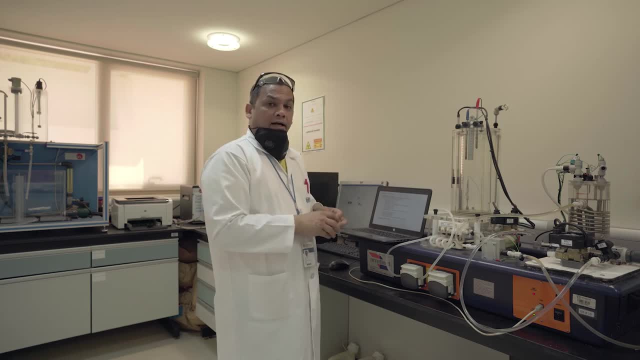 one. next is what i am looking for. remember, in the beginning i said i want to find out what is the best pid value for my system. so my controller that i need to use so that it is always maintained whenever you apply disturbance, it always maintain to my set point. so i want to find out the pid, the 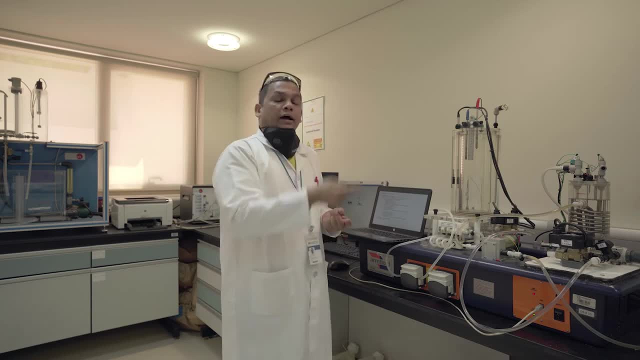 best pid value, which is what we have already done, using the matlab also, as well as using the sim link. so now what i have to do is i have to find the pid best value. remember, i have already done the part a and part b, in which i have varied the p about, i varied d, and i have all now acquired. 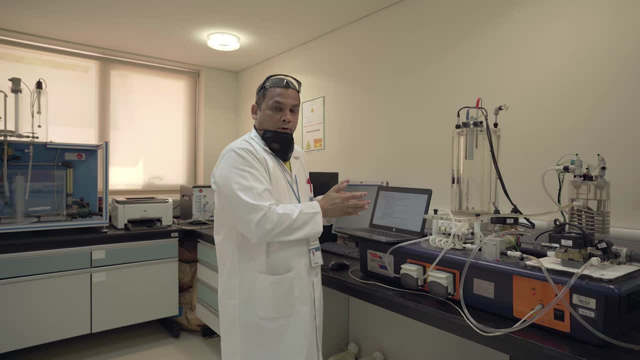 some knowledge that how the p and i and d individually impact my controller. so now i need to do is i need to start somewhere where the pid value should be, and how we do is called on and off method. so in an on off method, what i will do, i will put the control, i will activate the controller. 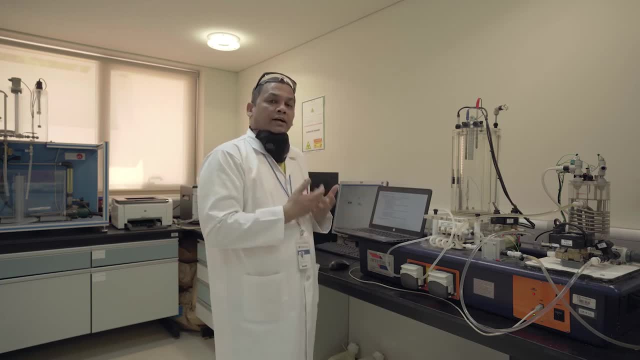 but put the value of p, i and d, so what it will do. the controller is on but it is unable to take any corrective action. so the the set point or desired variable. so if my pressure flow or temperature it may be varying between the lower and upper range, it's called on and off. on and off. so i will check that. 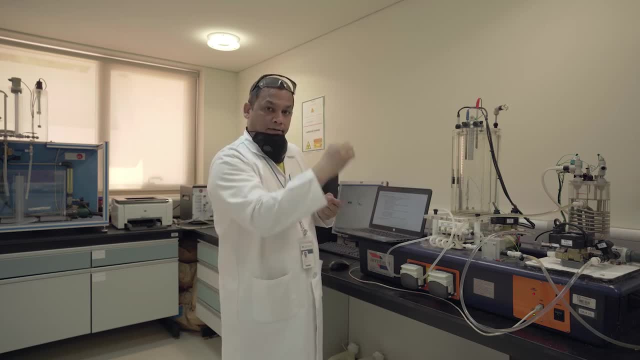 one. so the difference between the upper part and the lower part, the first peak and the first drop, this will give me y, and y will be basically the time it need to reach from the top to the bottom. it is made my proportional time. then i need i, i value. 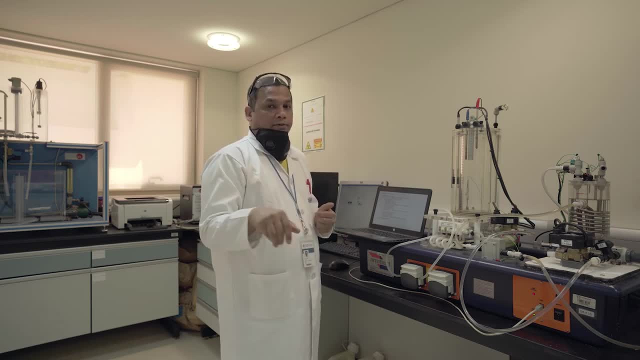 is usually p over three and the d, basically, is going to i over six. so this is how we can go and actually can find out the p basic value, pid, then this pid value. i am going to apply my control to see the response. it will not be the best, so i will then use my basic knowledge that i have just now. 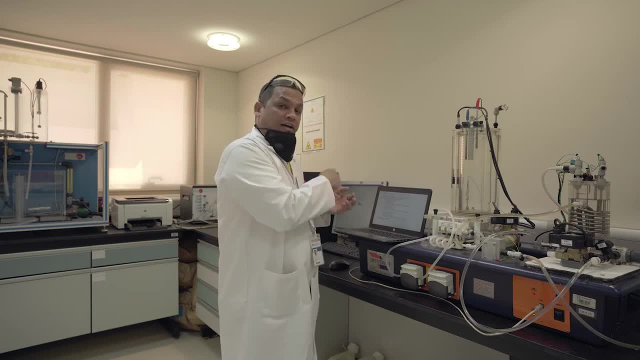 gained by varying the p and i and d. should i know that? okay, it is taking a long time to reach to the set point. so i will increase the i, or i will decrease the d, or i will decrease the i. so that's all about the experiment, everything that i summarized. so you are doing in two parts. 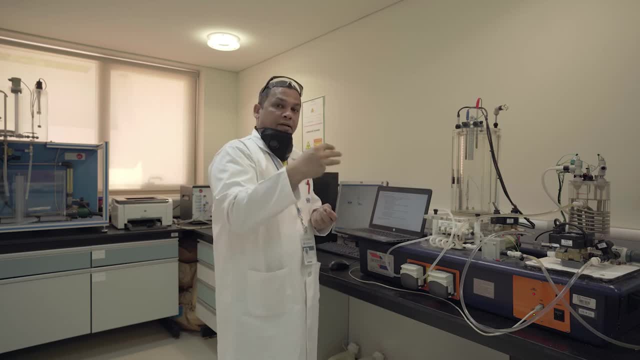 inlet about manual variable after manual variable. first you are changing p three times minimum, i three times minimum, d, three minutes, so that you study the impact of them. then you are going to do a on and off setting for the controller so that you find the base value. then this base value you are. 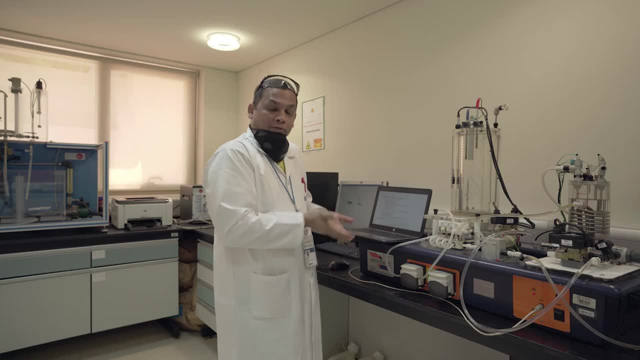 going to apply in the controller then see the response. it will not be the best one, so you need to just manipulate something. so i will change the p- decrease, increase, change. i increase, decrease, d change and see the response. when you find a very good, smooth response, the fastest that is your the. 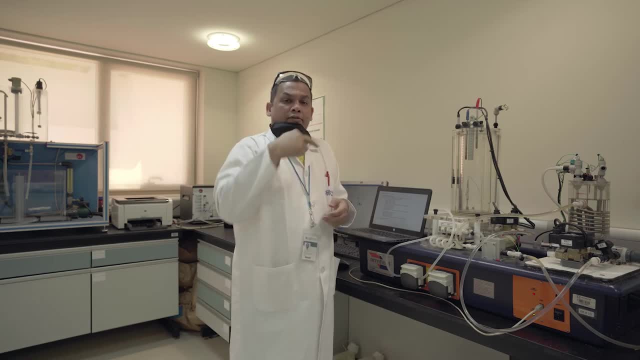 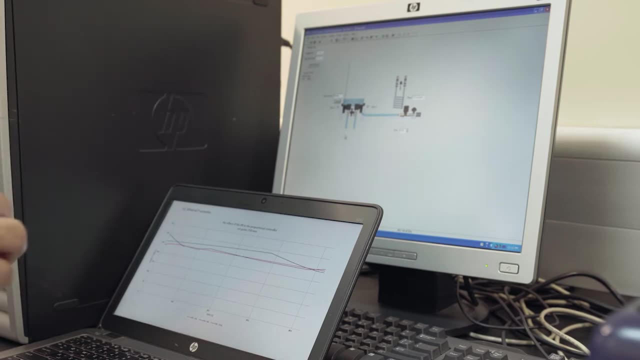 id value for experiment. one, when you want to control the level for experiment. two, when you control the temperature. three, when you want to control the flow. okay, so this is the first experiment, which is the level control. i want to control level in my tank. this one, which is the 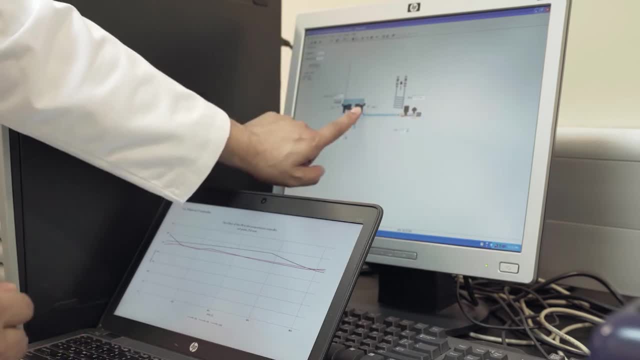 big tank we have already seen. in this one you have water supply coming in, so this is my inlet right now. i'm not manipulating that one, i'm going to manipulate the outlet. so my controller is here. if i put this is manipulated variable, then control will be here. 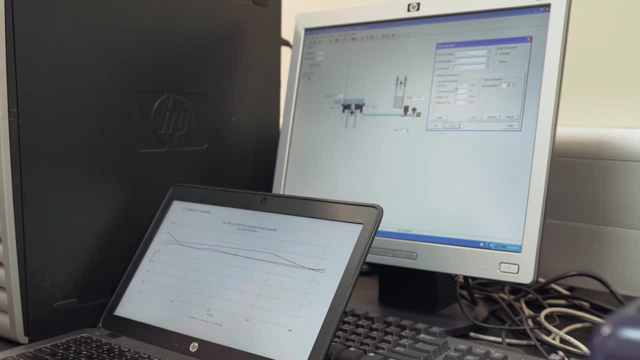 what i do. i will open the controller and you can see here this controller has a set point. so i will put what is the level i want to maintain in my tank. let's say i want 250 mm in my set and you can see there is a p value. i value d value. 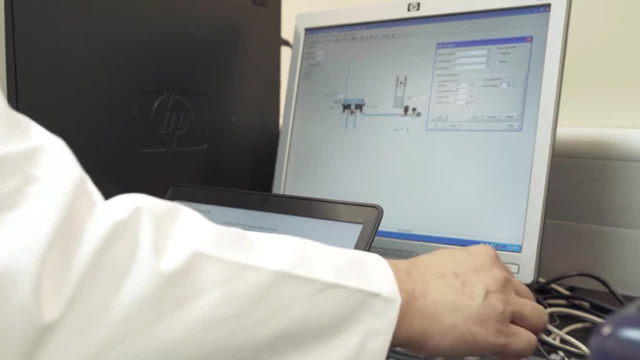 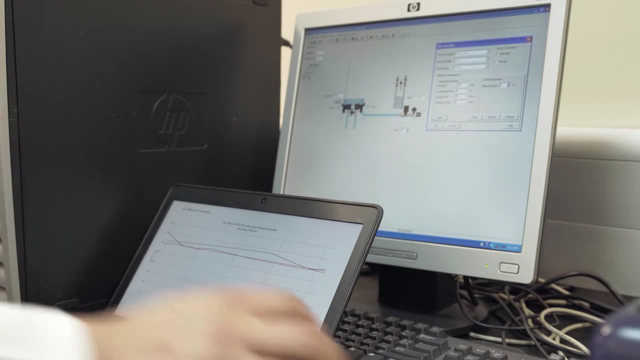 this is some value which i used last time so i don't need to do remember the first thing. first i have to do is keep the the d value 0 and i value 0. now i want to change the p value 3 times and see the impact. so i will say i will start maybe from. yes, the value can be 0 to time because 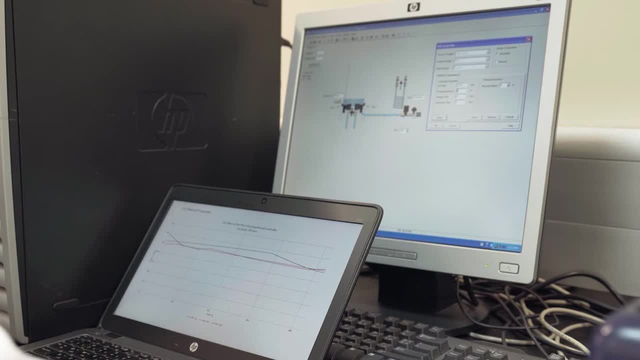 it's the time. so 0 to 100 or 200, whatever. so i will just say maybe i want 5 and i want to apply and i say, okay, this is the mode of operation. so automatically it will try to increase the level or decrease the level from manipulating the the psv valve here. so what we? 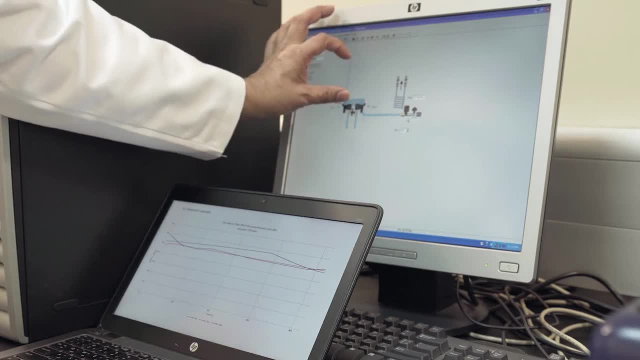 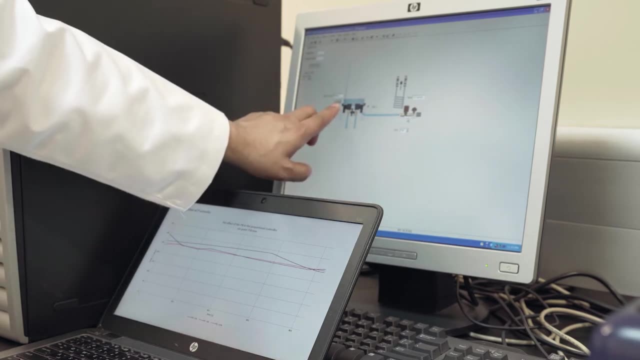 are doing here. you have the differential pressure, so it's measuring the height here, then sending the signal to comparing with set point. sending to controller control is then saying that, okay, this level is less than the the set point, so you need to open the more so this more will come and 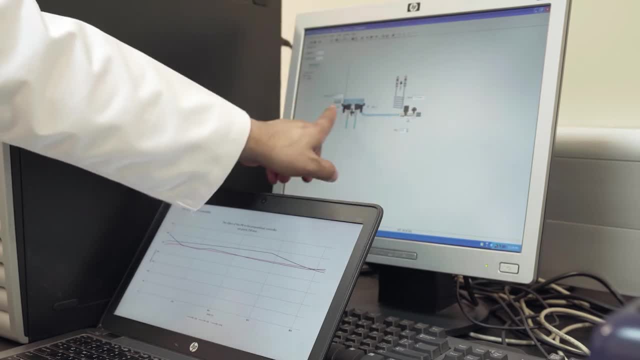 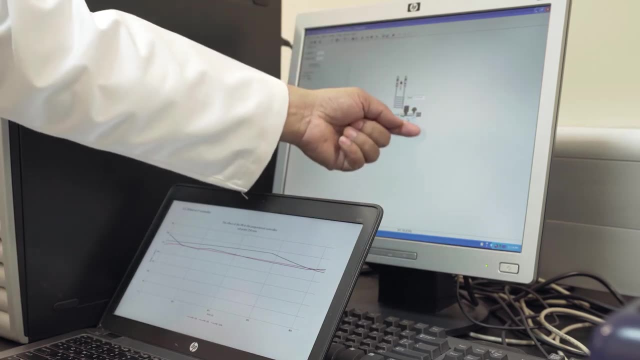 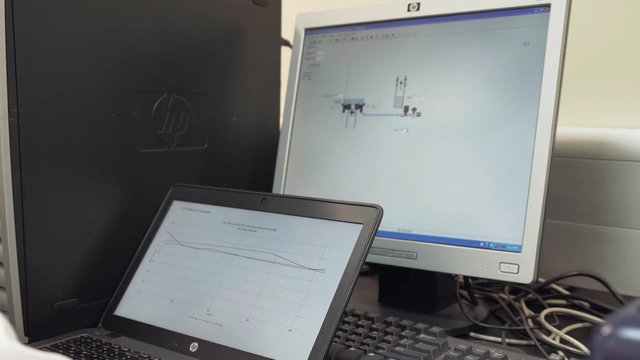 level will rise. okay, uh, or it's: uh. if it's the level is already more than what is set point, then it will say that, okay, can you close the wall so that the level can be maintained? and in this way i am, i'm plotting this one and then recording the data and seeing the, the plot here, uh, so this is. 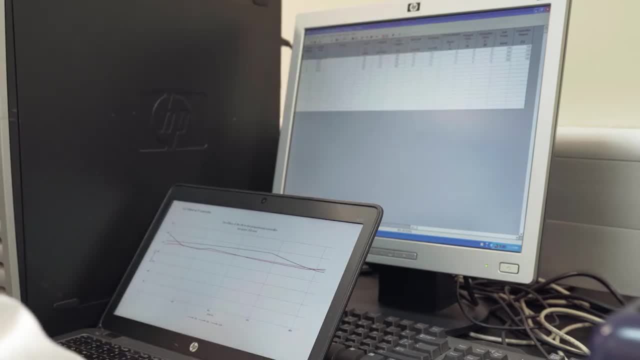 first value of the p. once it is supplies, i stop it and i can go back to my controller and change it to another value of the p. here now i will say that p value is 50 and apply and see the response one more time and then again. 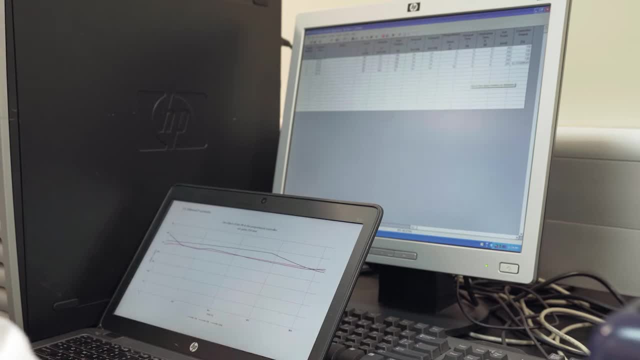 start recording the data here. you can see the plot here now, second time, then third time. so all the three, minimum three, as i said, uh we are going to do and then we can plot three together. so you see here three plots. i have uh with different values of p 1, 5 and 15 and you can see. 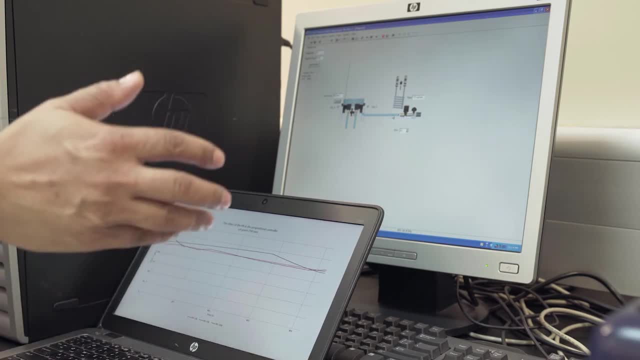 here. uh, from the three plots you can see that the value of the p is 50 and the value of the p is 100, and the value of the p is 50 and the value of the p is 100, but, um, as you increase, uh, you, you say there: 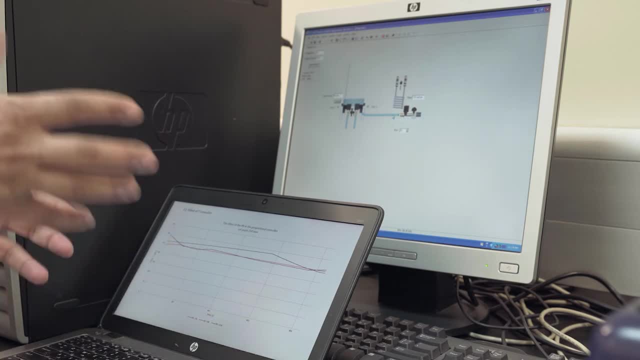 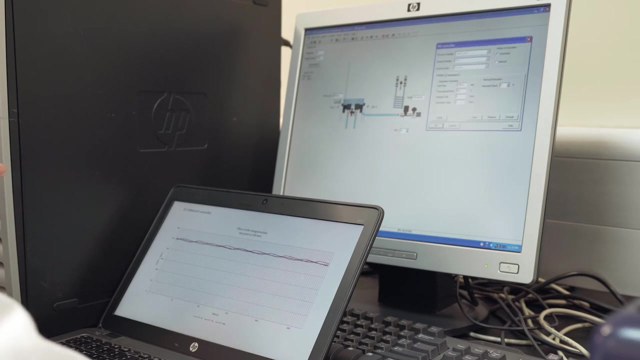 is a better response. okay. so in this range i i can somehow see that. okay, if i will increase the p then of course i'm going to get a little bit better response than this one. so this serves me in the background for the p. now, same i'm going to do for the d, so to do the first integral times, okay, i'm. 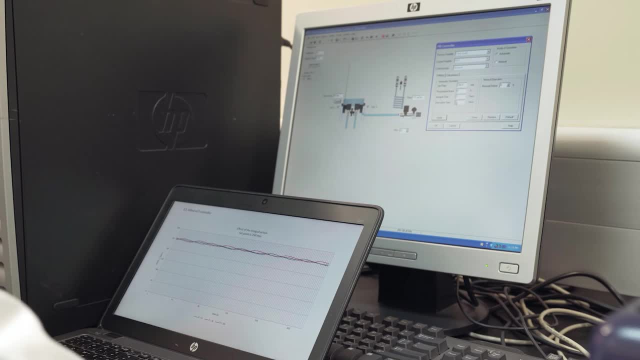 going to fix this p value. p cannot be zero, okay, so i am going to fix uh the p here and i will forget and change the i uh three times one maybe, let's say um one second, then five second and 15 second and 20 second, like that, and apply and see the controller response. so the level response i am 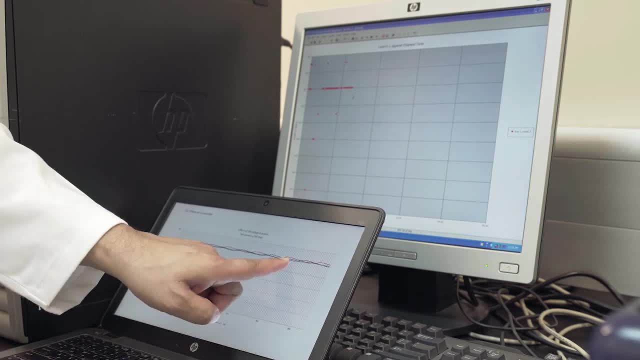 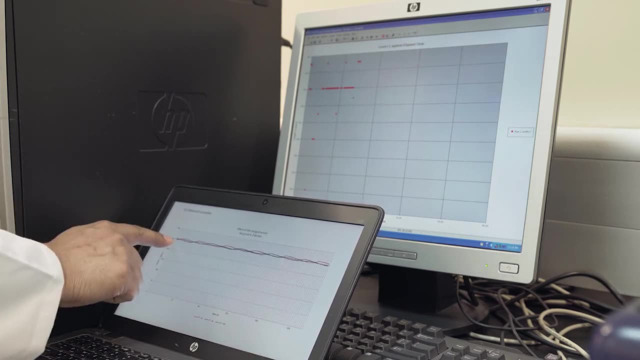 watching from here. so three of them i plotted here. now. this is the the integral time impact, and i see that one uh, they, they basically uh work in a very good tandem. um, if you see the the blue one, it will have uh more fluctuation. uh, which is the this one, uh, the high value of. 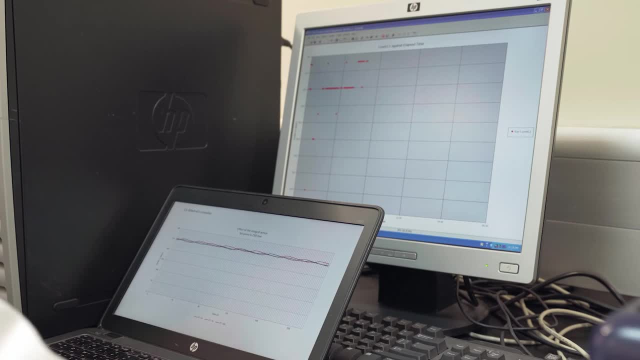 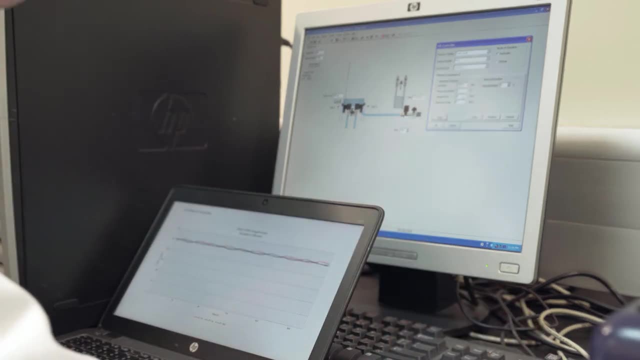 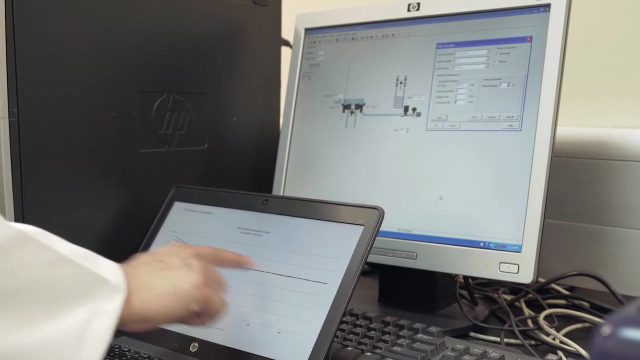 i. that means that i try to keep the level of i- integral time- less. then i go to the third one, which is the derivative time. so i will fix a value of d here also. i also here and now, three times d, so three times. when i change the value of the d, i get this plot okay. so this will help me. what is? 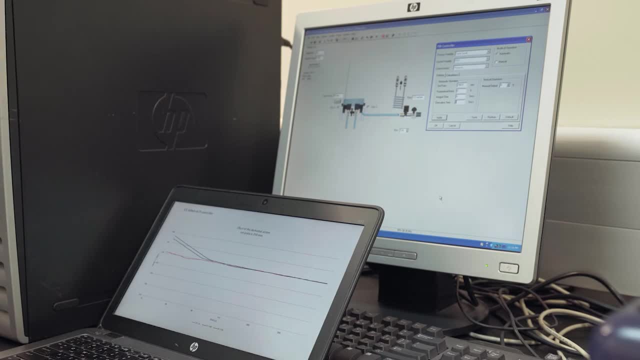 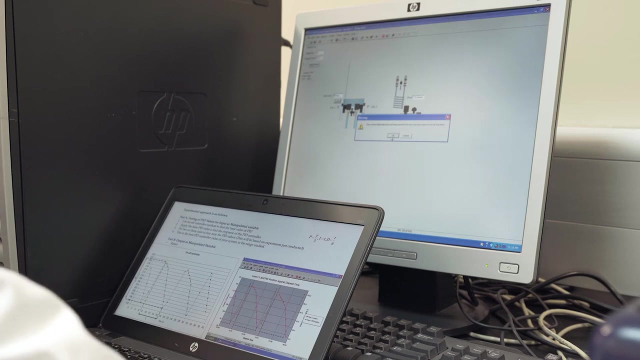 the impact of p, what is the impact of i and whatever d when i am using my inlet as manipulator variable and from there then i will go to do the same thing again for the outlet as manipulator variable. so i will choose the new experiment that i have to do and where i am going to do the level as outflow, as 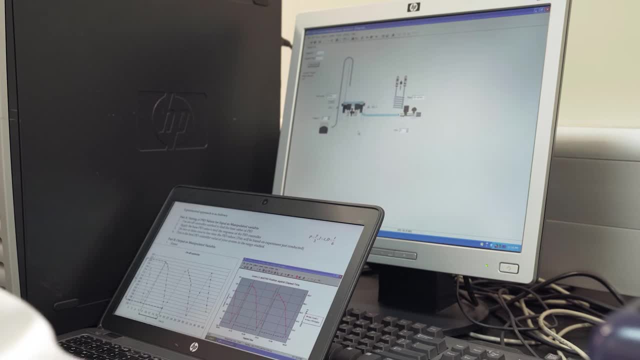 my control variable. so you can see here i have this tank, another one here connected here which i am going to use as a control variable. so controller is going to control. it is showing here what is the level. this is my set point and this one. so i do the same p and id three times. okay, 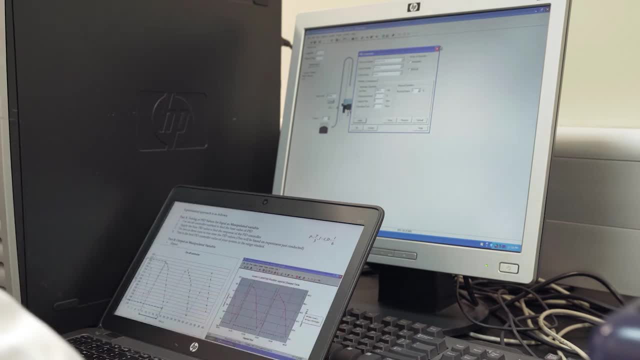 the three values of pd3 by 53d. then that is my background and then i am done with this one. now i want to find out the pid best value of the pid. so i will go to the controller and i will put 0, 000 here and i will put automatic so that it will automatically try to control. so the controller is. 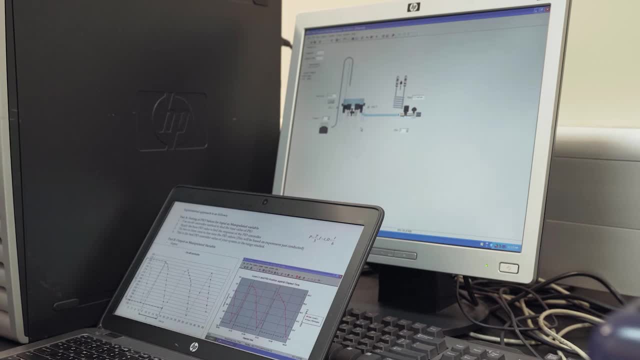 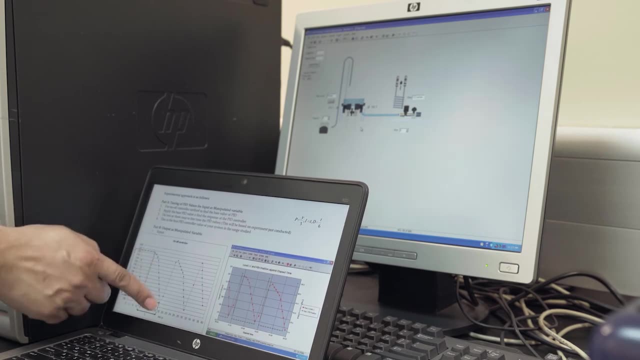 trying to do something, but we cannot do any correction, so it cannot apply anything. so you will see the value of the level rising between uh, upper minimum, maximum and minimum. so this is how we can see here, and from this graph i am going to get my base value of this particular low. 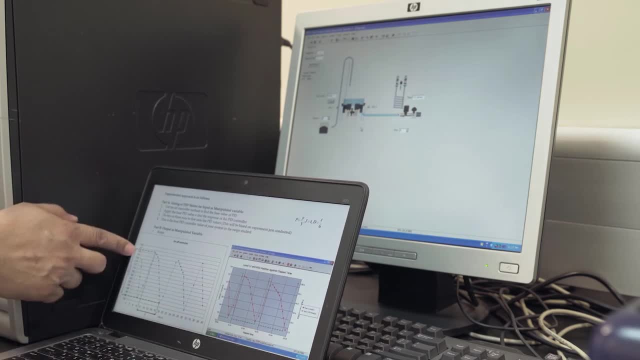 to get my base value of the pid. i see this is the y. okay, this is the highest value, this is the lowest value. so the, the, the y over 3 will give me the the time. so right now i can see here: this is 194 to 20. so i just subtract so it's like around 2- 8. so it's like 30, 30 divided by 3 is 10, so p. 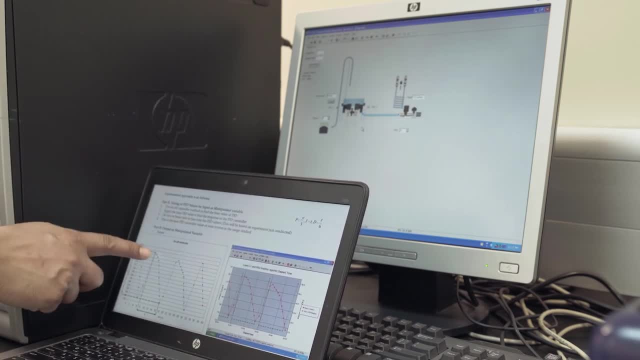 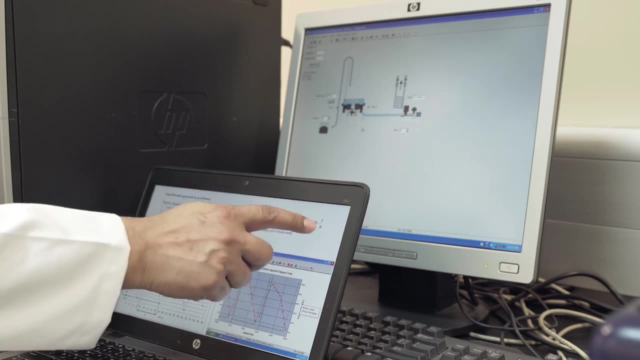 value time. reference value p is 10 and then time it takes to reach from the maximum to the minimum is going to be the t, and t is my integral time. integral time is 8, so 16. so it's 8, 8 seconds, and 8 over 6 will give me the id. so this is how i got the pid. now, this pid i am going to apply. 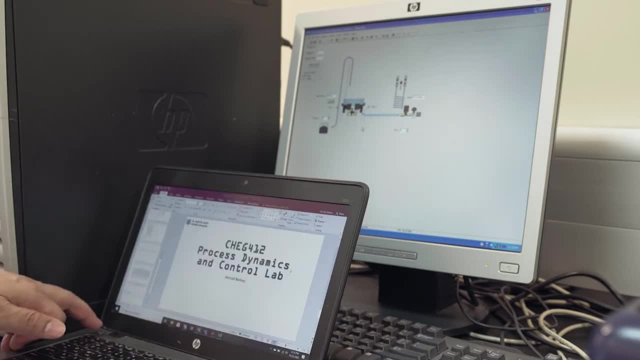 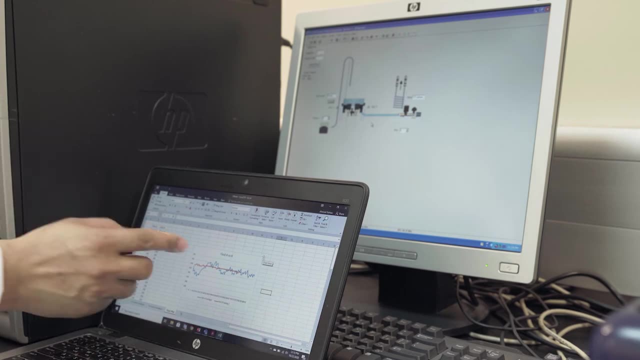 and try to tune it. so then i will uh, tune it to get the best value which is here. so i, in the controller, now i am applying this pid that i got from the on and off setting and seeing the response. so i- the blue one is the first response i got and i saw that this is not. 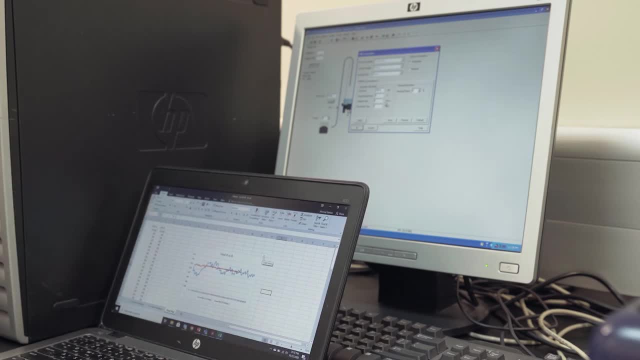 valuable. very good. actually it is better, but it's not good, so it can be improved. so i change the p value, i change the i value, i change the d value and i find that this red line is the best pid value for my controller. so to maintain this level, this is my best pid value for the controller. when inlet has. 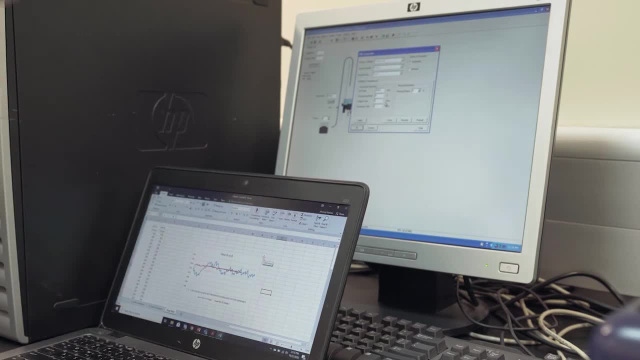 manipulated value. so i'm going to repeat the entire experiment again for on and off, to find the pid. then apply the pid into this one and then see the response. to find out what is the uh, the, the base value, base value. apply and get it for this one. so this is how you can do the experiment. this is: 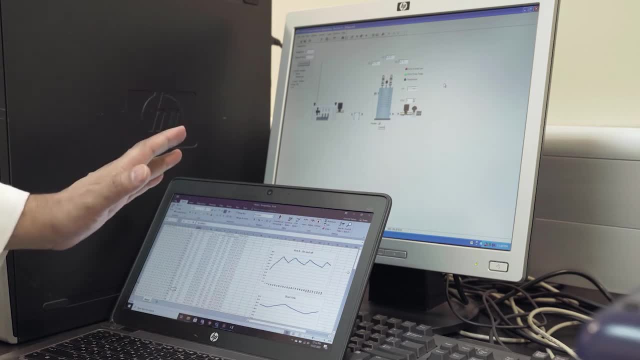 the entire experiment. now this is our second experiment, which is the temperature control in the tank. so you can see here the tank in which i have the heater. again the same. you two parts. first part is inlet as a manipulable, second part as outlet, a manipulable variable that you want to. 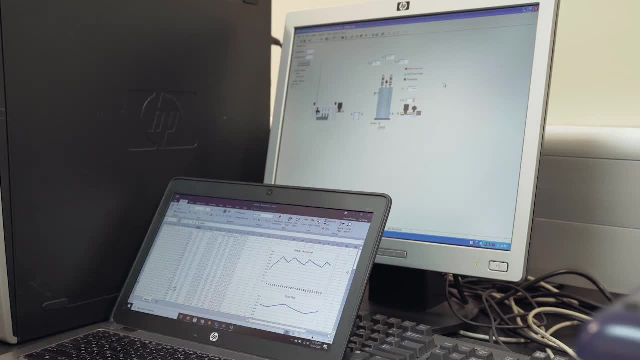 do, of course. inlet is here the power, how much power you want to give. the outlet is here the flow. so the more flow you are taking is like less power you are applying. so the inlet and outlet variables are there. so two parts. first, remember what i have to do. i have to open the controller and set it. 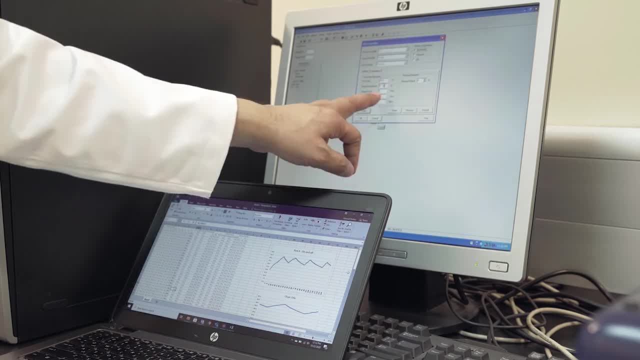 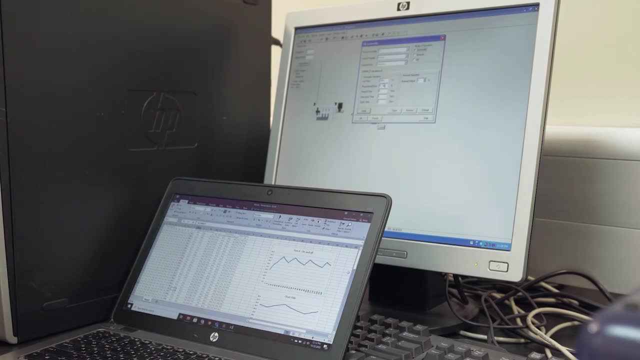 automatic. set my desired temperature- right now temperature is 30- and then start with the three value of the p and while keeping the i and d value zero. so i will know that how the impact of the p will be. then i come and fix the p value and put and three different value of i and see the three. 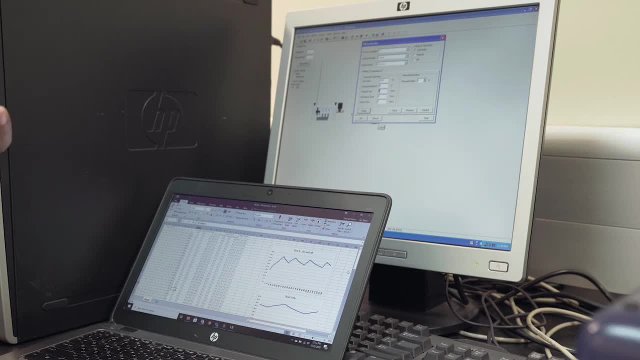 different plots and see the response of that one and how the three value of the i will have role in that one. then fix the i value and the p value, both, and then change the i, the d value, three times and see this one, both for inlet, as manipulable output, as manipulable, which may be power, which may be the flow. 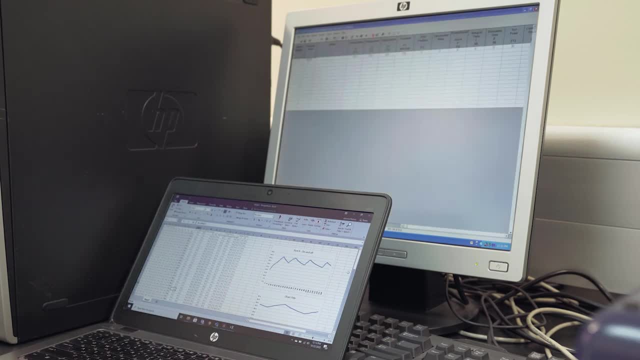 okay, so you are doing the same. you are report, recording the data. so, same set of data, same thing with this one. now the next thing is: we'll remember, we want to go and find out the pid value. so, to find the pid value, what i'm going to do is i'm going to do the on and off so that i can get. 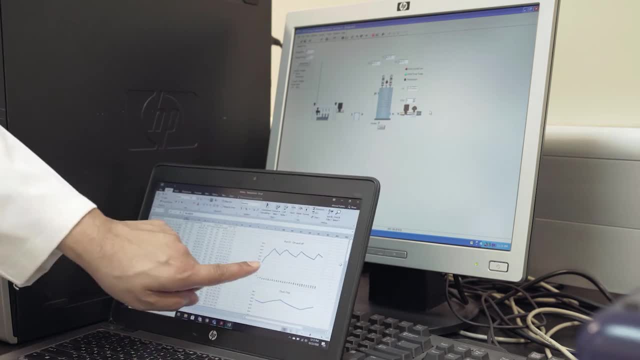 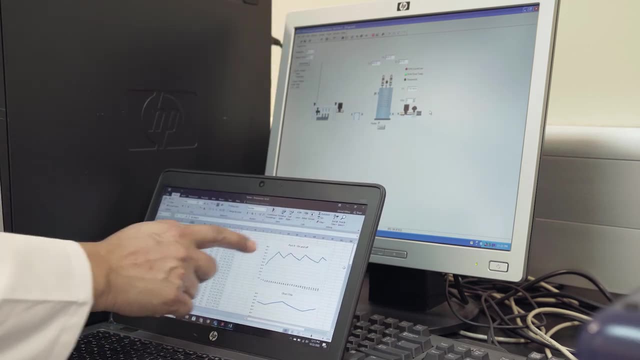 the basic value and then apply so. so when i do the on and off, i get a plot like this: you can see it's. this is fluctuating between the lower minimum and maximum. so i can see: when the set point is 30, the maximum is going 45, the lowest it is going around, uh, some 15 degree or so. so again what i do. 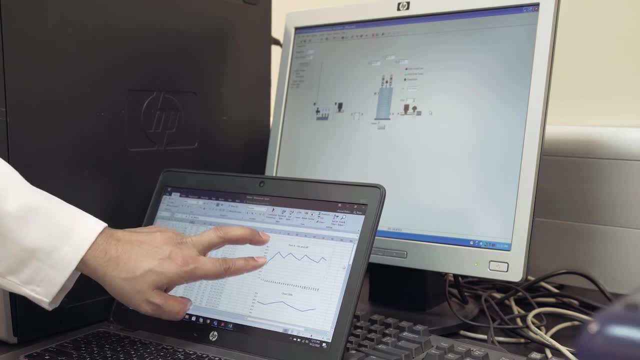 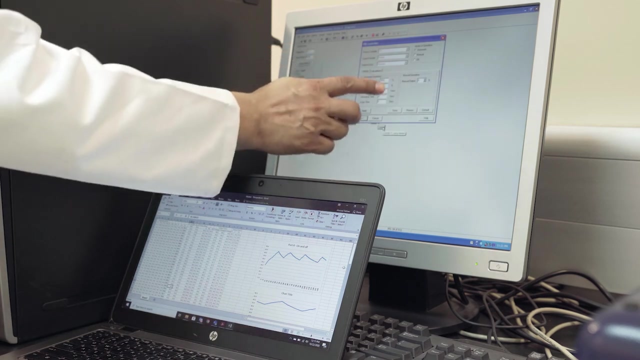 is y, the difference between maximum and minimum. so y over 3 will be p, then time it takes to reach to go from high to minimum will be the, i, i will be integral time and i over 6 will be my derivative. so i got the pid value. now, this pid, i am going inside the controller and applying the p value and 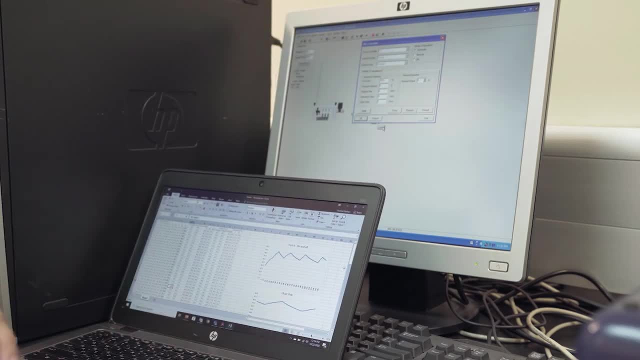 d value which i have got now from here, and then i can see here how the controller response looks like this one will be. it's not very smooth. then i try to change the pi, i try to change the d and then i get the the best value of the pid, of course, uh, when in letters are maneuverable, when outer 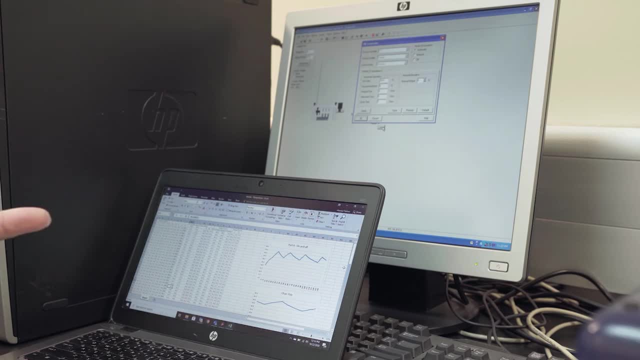 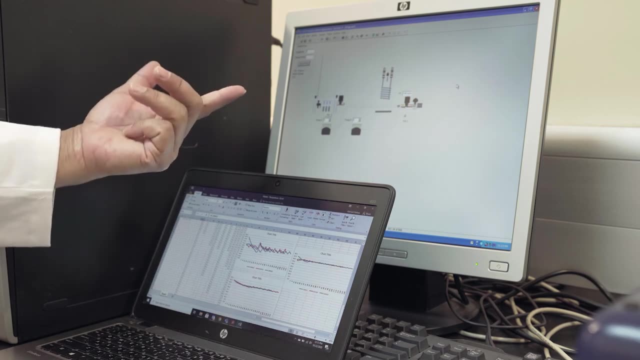 variable, variable, and then i can see that whether which one is easy to control, should i control the inlet or should i control the outlet? this is the experiment number three, which is the flow control. so again, i want to achieve a desired rate that i need. so it is no different than the other two experiment. it's the same. uh, what i have. 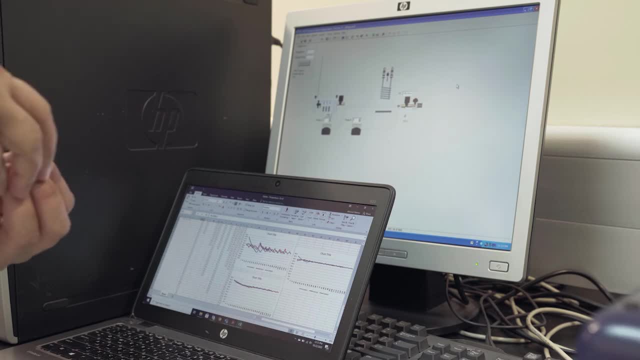 to do? i have to use uh orifice meter we have, so it's a measuring device that measures the flow. send it to the controller controller takes the action. now to take the action, you need the p and id value of the controller, which is what we can see here: uh, in my flow, uh, so what i will do? the